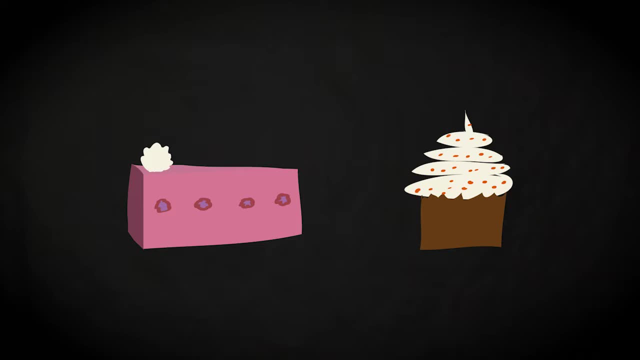 panel is to decide which of two candidate pastries would be most suited to become the next pastry of the month: The one with orange, mint and cream or the other with strawberry chocolate and a crunchy crust. The procedure is simple. After tasting, each panel member assigns a score between one and 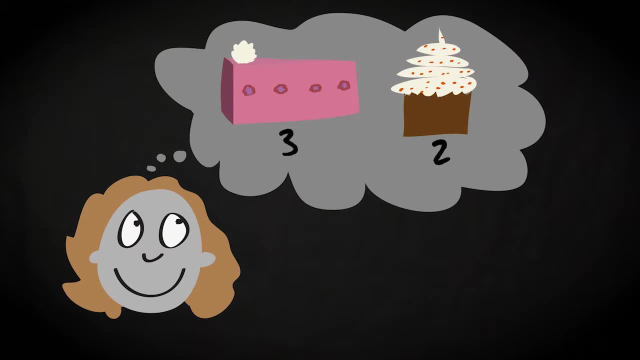 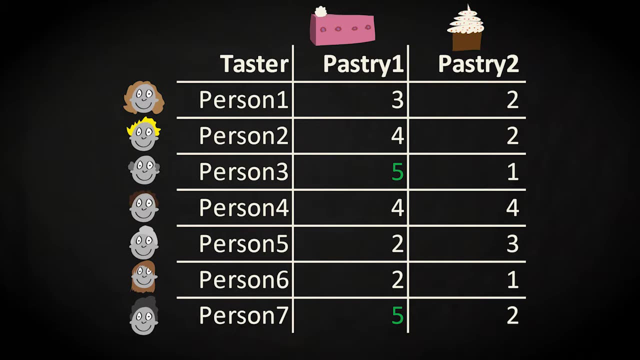 five to express how much he or she likes that pastry. This is the result from the panel. As you see, some members clearly prefer the orange mint pastry, whereas others would go for the strawberry chocolate one. So how to analyse this data? Let's start by translating the practical question of finding the nicest pastry into a statistical 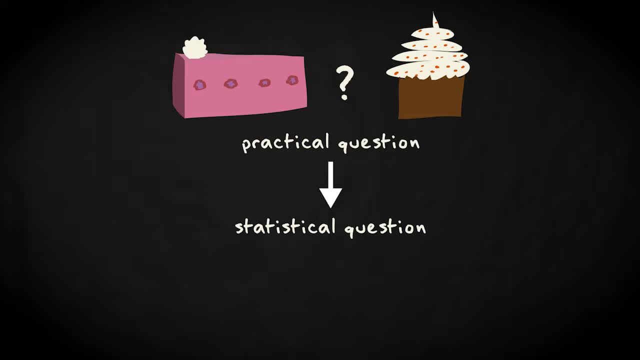 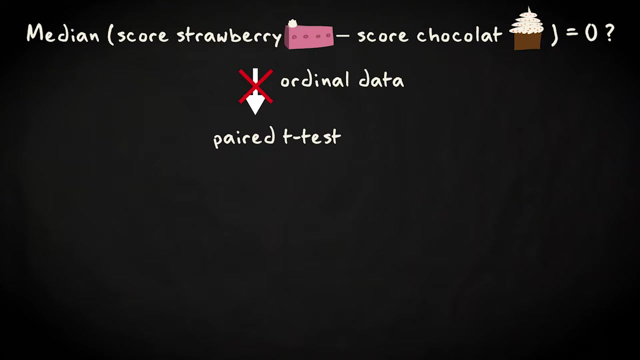 one suitable for hypothesis testing. The question becomes: is the median of the differences between the pastry scores different from zero? It is a two-sided test. You cannot use a paired t-test because the data is ordinal. On the other hand, you could use a signed test, but then you would throw away some of 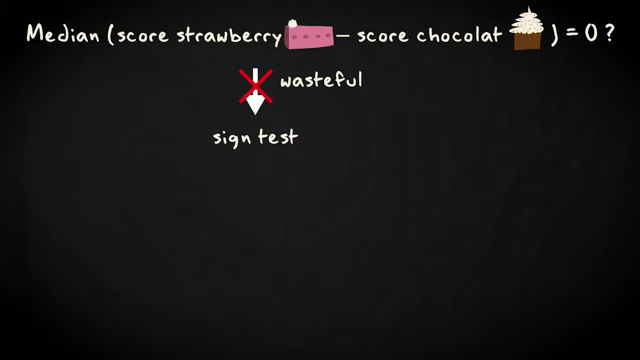 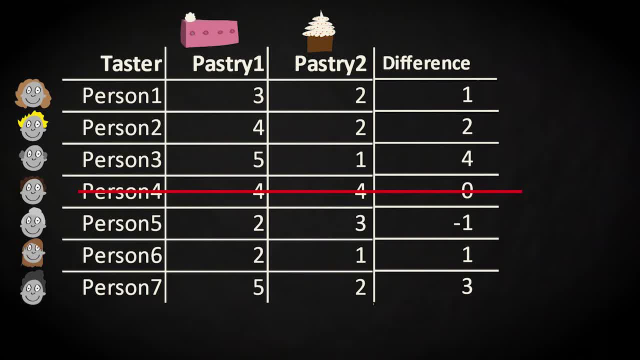 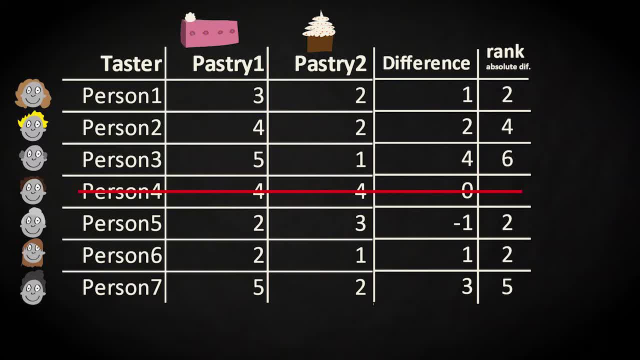 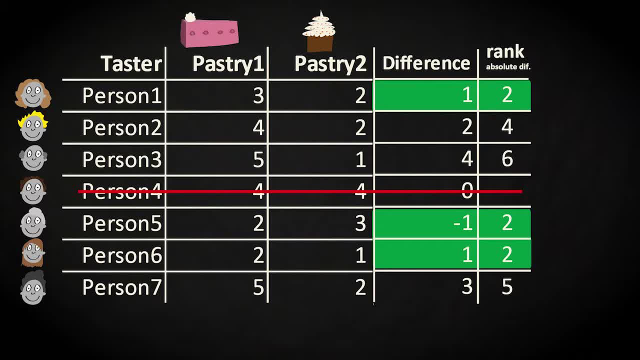 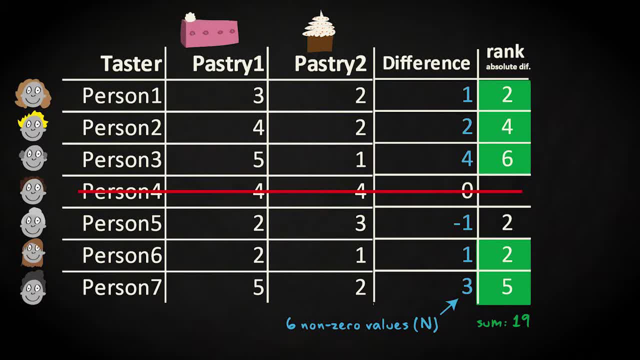 the number of values with non-zero differences. The value that you've calculated is the Wilcoxon Rank Sum statistic, often abbreviated to W. The bigger the value of this statistic, the less likely that there is truly no difference between the average scores. 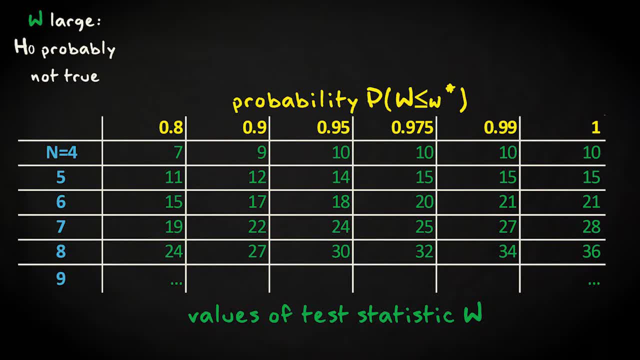 By using accumulative probability probability table or software, you can find the probability of encountering a given value, W or higher, with n non-zero observations. Because we are in this case interested in a two-sided test, this probability should be doubled. The pastry tasting example has illustrated the signed ranks test for a case with paired. 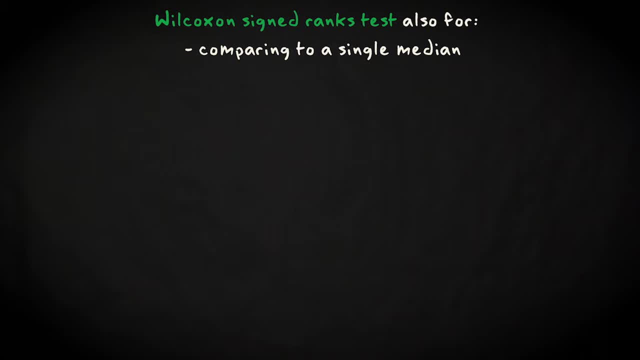 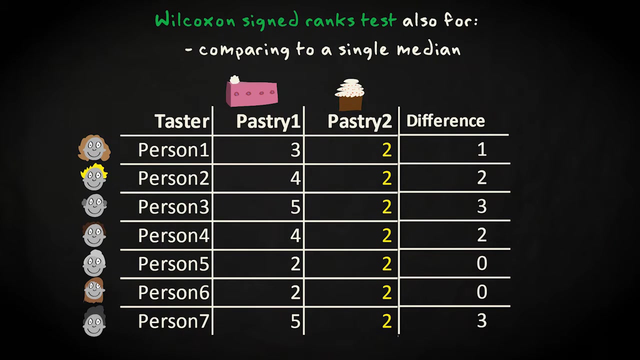 data, But it can equally well be applied to a situation with a single sample where you compare scores to a theoretical median. You are then testing whether the observed median scores are different from what is expected After replacing the values in this column with a theoretical median. all the calculations 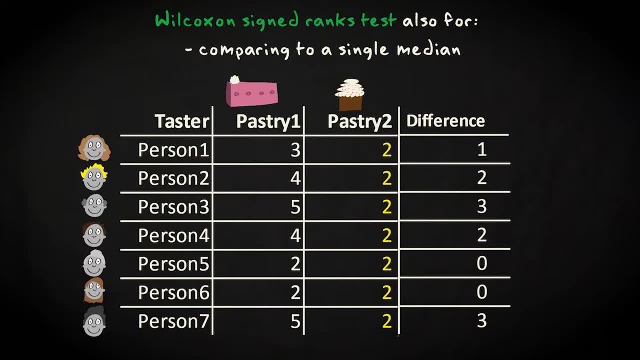 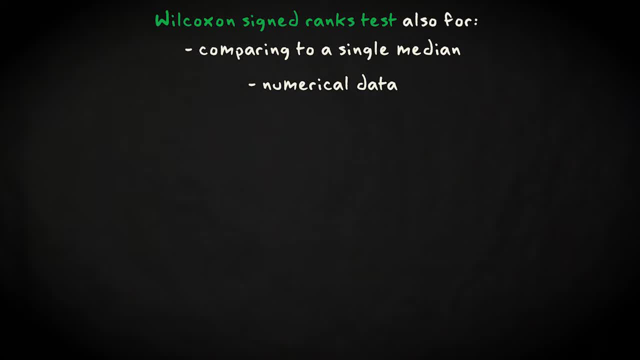 are the same Without any changes to the method. the signed ranks test can also be applied to numerical data. If you have paired numerical data, you would subtract the values per case and then proceed as in the previous example, by ranking the differences And with a single sample. you can then compare the values to a theoretical median. 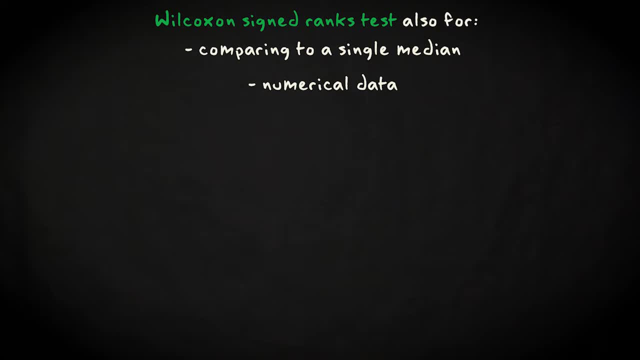 The power of the signed ranks test is quite high, almost approaching that of a one-sample t-test. A major strength of the signed ranks test in comparison to the t-test is its robustness to outliers. But a minor weak point is that it does rely on the assumption that the population distribution. 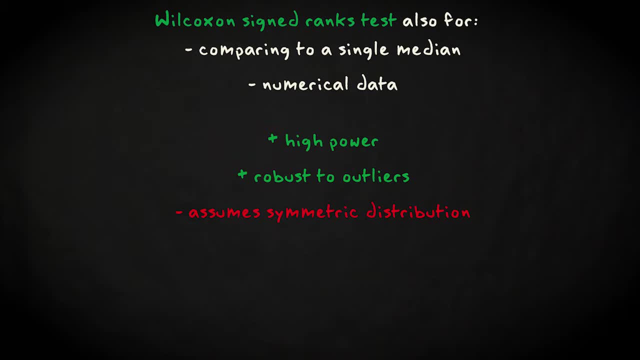 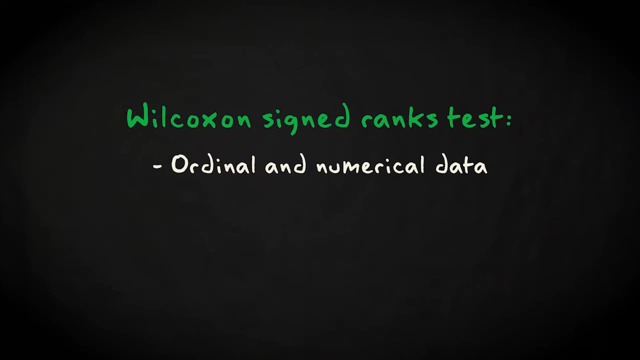 is symmetric, one that is difficult to check, especially for small sample sizes. Let me summarise: The Wilcoxon signed ranks test uses data that is ordinal or numerical and assumes that these are independent and identically distributed samples from a symmetric distribution. 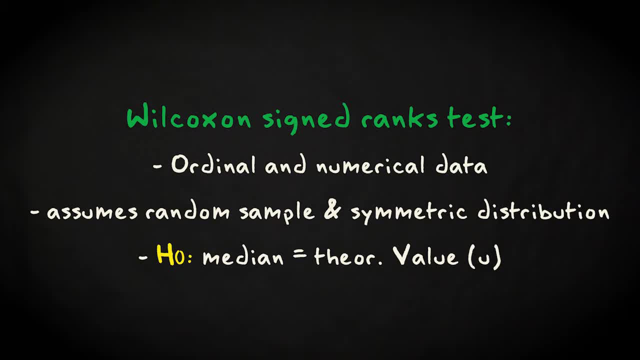 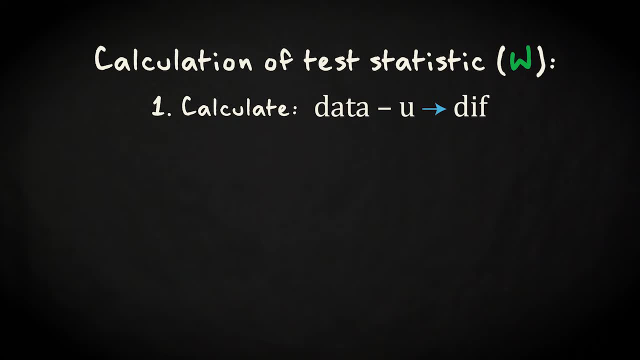 It tests the null hypothesis that the population median equals a theoretical value. The test statistic is calculated in four steps. First, the differences between the data and the theoretical median are calculated. Second, cases with a difference of zero are removed. Third, the remaining data are ordered according to the absolute values of the differences. 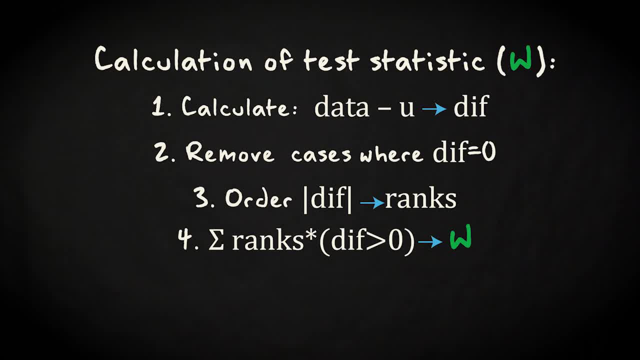 And fourth the ranks for the positive differences are summed. This test statistic is compared to tabulated values. A special case occurs when you have paired data. In that case, the data values per pair are subtracted and then treated as a one-sample.